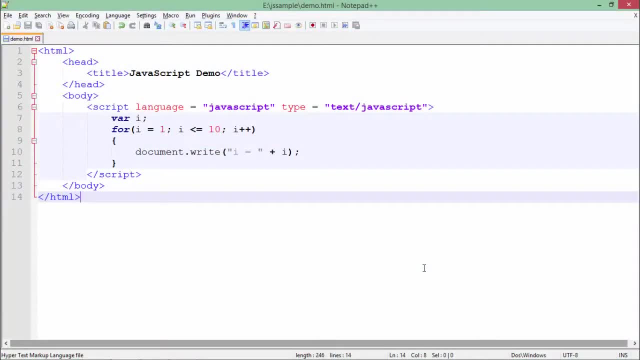 So in this program I have written a for loop which is starting from 1 and will run till 10.. So if I will execute this particular loop, obviously I will get the numbers printed from 1 to 10.. So let's check it out first. 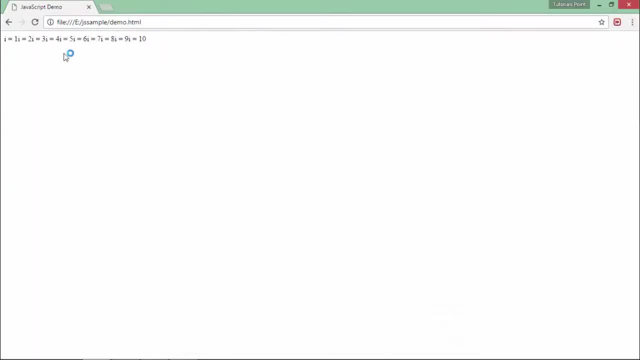 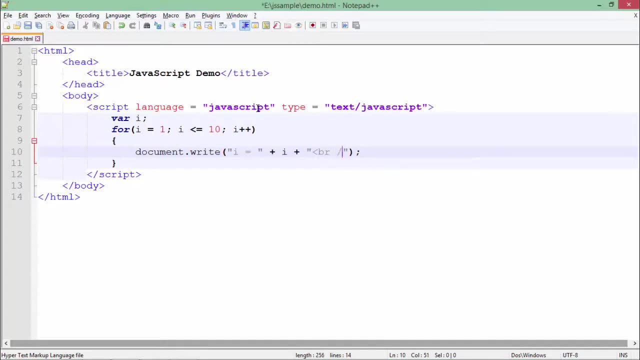 So here in the browser, I will open this particular file and you can see Alright 1 to 10.. Let me do the line break as well along with that. So, br, along with this, Alright, let's refresh. 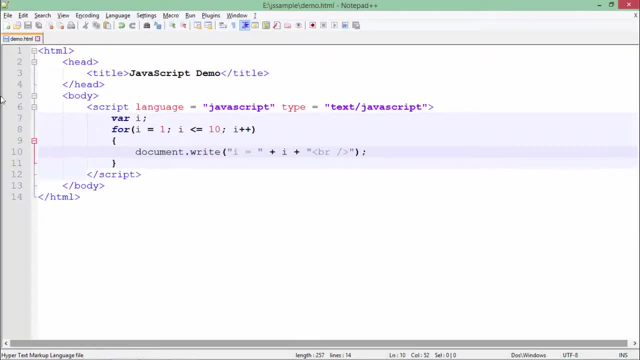 Alright, so this is my desired output. But if I will introduce any loop control statement in that, So obviously the output will be differ. So let's execute that. And here I will pass a condition like: if i is equal, equal to 5.. 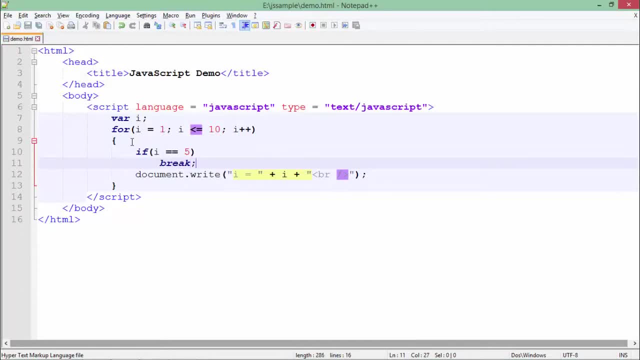 Then I will say break Alright. so here, as I discussed what this break statement will do, It will terminate the loop. So when i will become 5, the loop will be terminated And obviously the execution will be stopped out there itself. 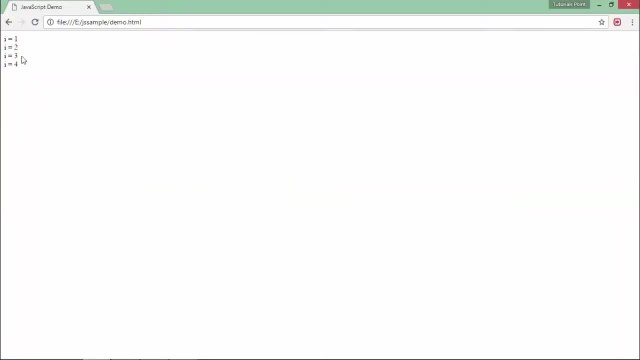 So if I will execute, you see, Even though I have written the loop from 1 to 10. But since I have introduced the break statement when i was equal to 5.. This particular output is looking like: this Means it will just running for 4 time. 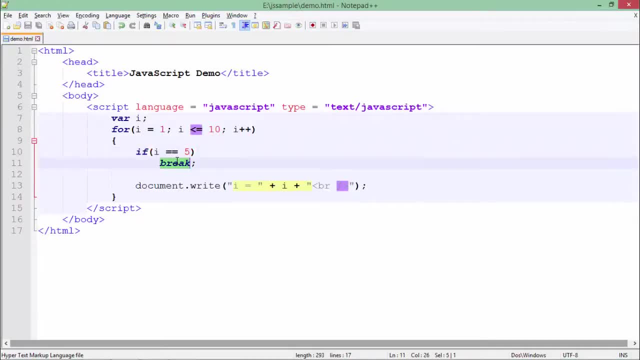 1,, 2,, 3 and 4.. So this is about the break And the similar thing it was doing at the time. we introduced this break statement in this switch Where, when any of the case was satisfied, The execution was terminated because of this break statement. 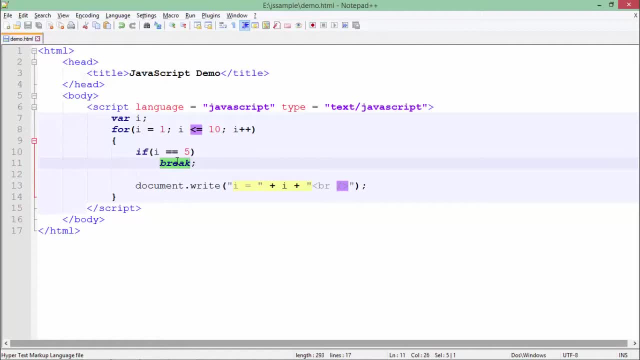 And none of the case was checked inside, that switch again. But if, apart from this case, Apart from this break, I will introduce a continue statement. So what this will do, It will just skip the cycle, Means I am running this loop from 1 to 10.. 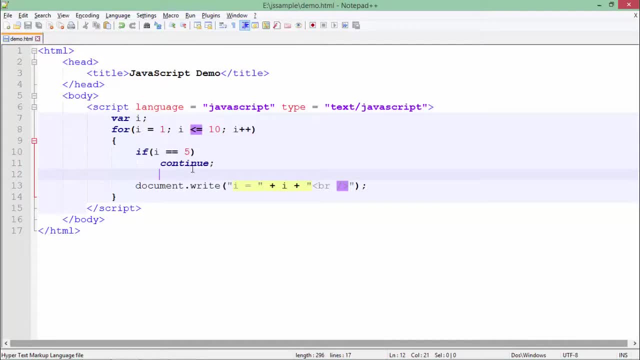 So if I will say i is equal to 5., Then continue. So that means this loop Means this particular statement will be skipped when i was equal to 5.. So this is how the output will look like. So, as you can see,